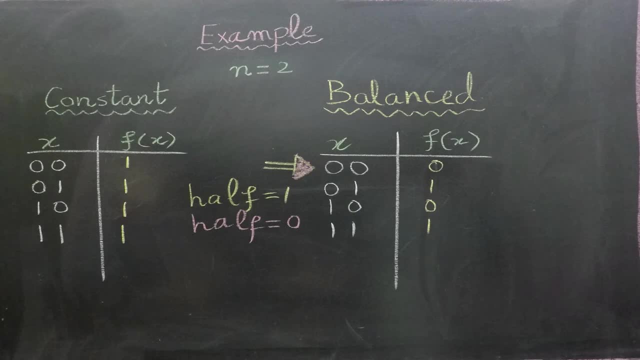 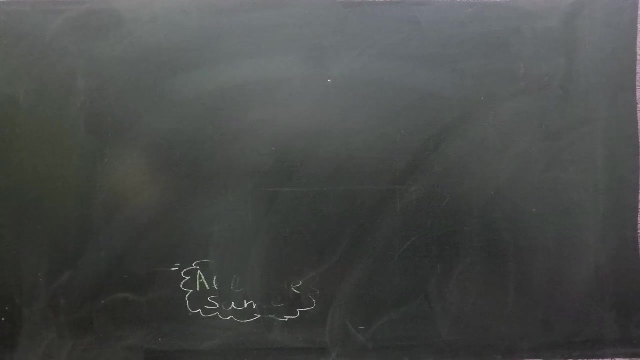 long as they represent half of the total inputs. Thus, when half of the inputs are the same, the function is balanced, whereas for a function to be considered constant, all inputs must produce the same output. How can we solve this stated problem using classical computers? Well, on a classical computer we must examine one more than half of the total. 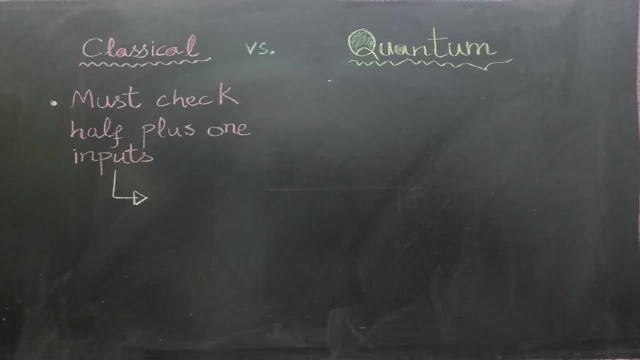 inputs. Thus the total number of inputs we must examine are 2 raise to power n minus one, plus one more than 0. So the new rumors are true. Moreover, for one additional input, This implies our time complexity of O, which is exponential. 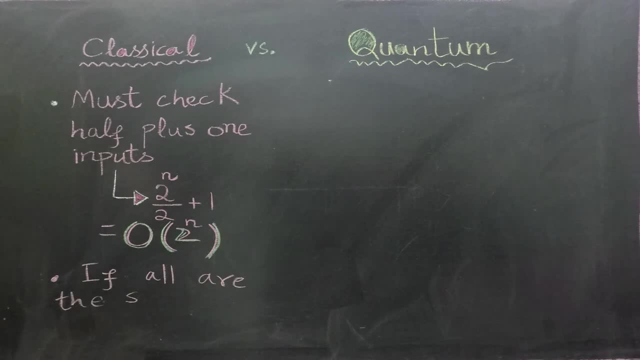 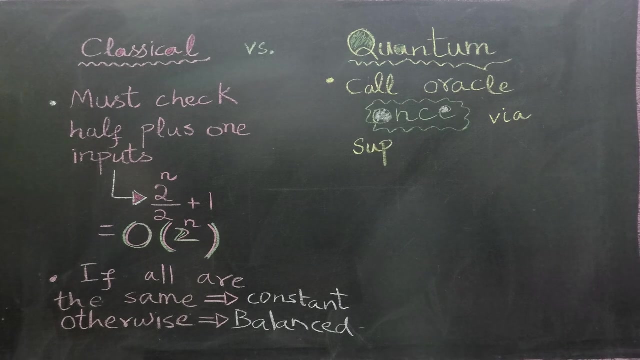 If all of our inputs produce the same result, then the function must be considered constant. otherwise it is balanced. In contrast, on a quantum computer we call the oracle only once. This is due to the magic of superposition. Thus, on a quantum computer, we are able to. 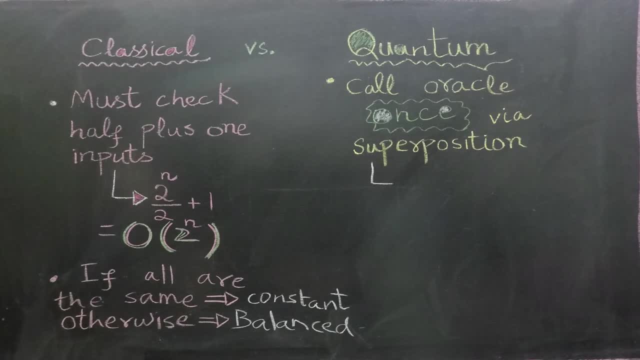 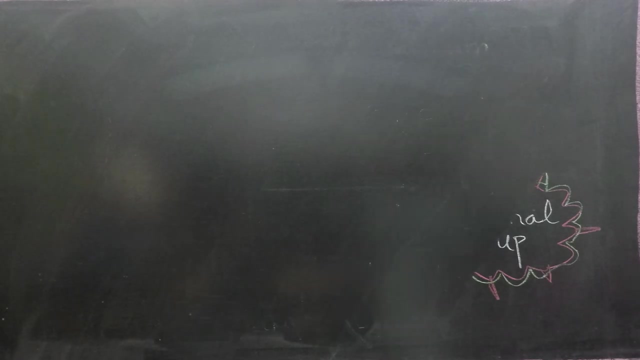 solve the same problem in O time complexity. This represents an exponential speedup compared to the classical approach. The quantum circuit of Deutsch-Hauser algorithm starts with two registers. The first n-qubit register is initialized with ket zeros and the second single qubit. 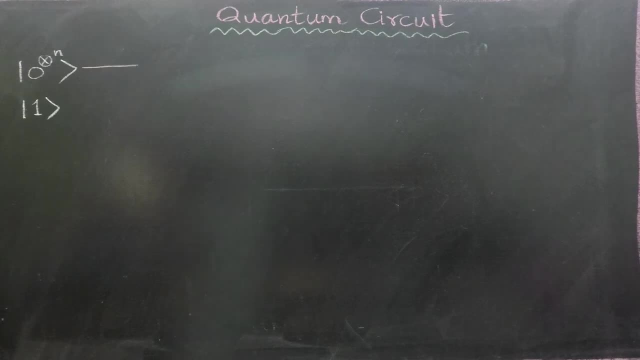 register is initialized with ket 1.. Then Hadamard gates are applied to both registers, creating equal superpositions. The superposition of all the inputs and ket minus is then passed to the UF gate. If the input to the UF gate is ket X and ket Y, its output will be ket X and ket. 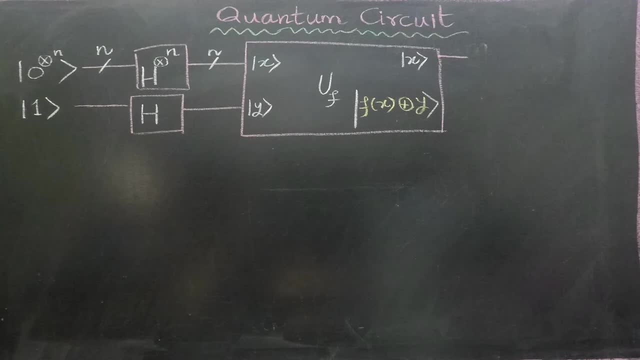 F of X XORed with Y. Finally, the first register is subject to Hadamard gate once again and measured. If our measurement results in ket zero, Then the function f is measured and got to the is constant. Otherwise, it is balanced To understand the algorithm, the quantum circuit. 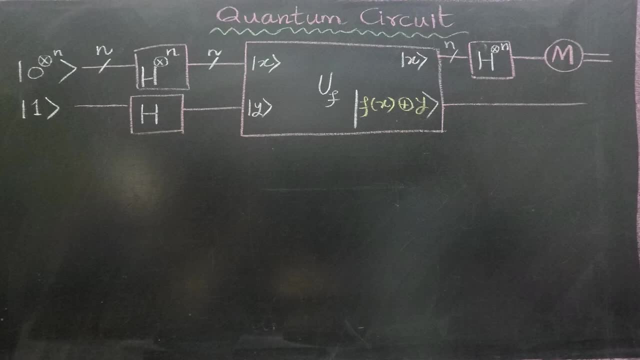 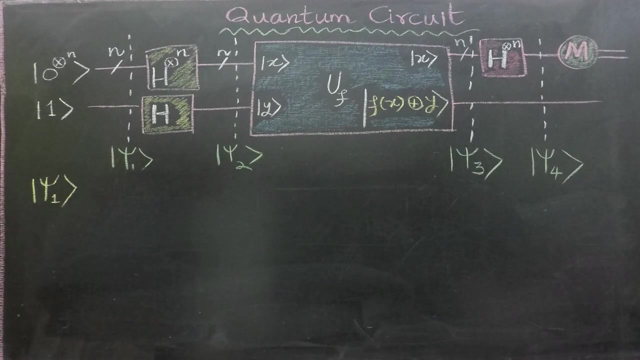 is divided into different stages. The first stage is referred to as ket psi 1.. The second stage as ket psi, 2.. The third stage as ket psi 3 and the last stage as ket psi 4.. Ket psi 1 is equals to ket 0, tensor product with ket 1.. 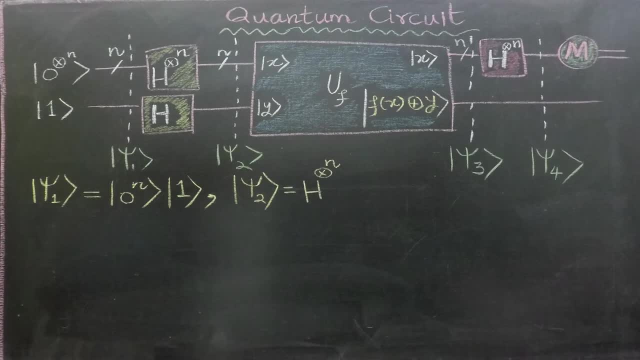 To calculate ket psi 2, we apply Hadamard gates to ket psi 1.. Thus ket psi 2 will be equals to 1 over square root of 2, raised to the power n times the summation of all the n qubits combinations. 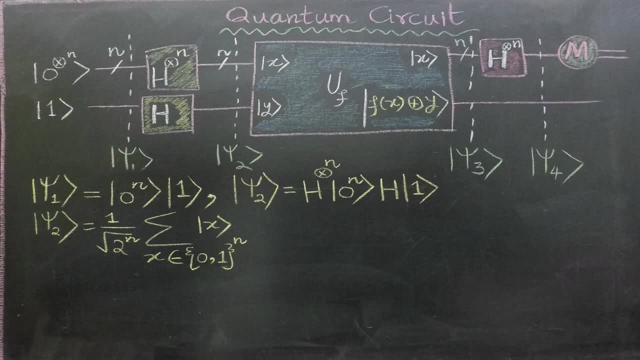 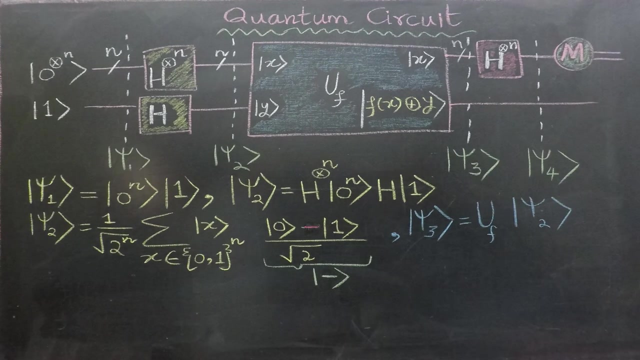 Applying a Hadamard gate to the second register will gives us ket 0 minus ket 1 divided by the square root of 2.. Note that this is referred to as ket minus. To calculate ket psi 3, we have to apply UF gate to ket psi 2.. Remember that if the input 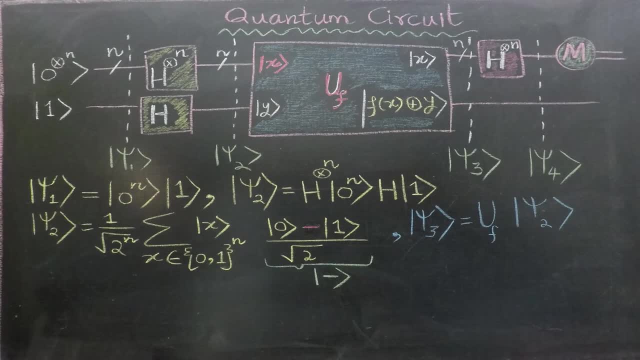 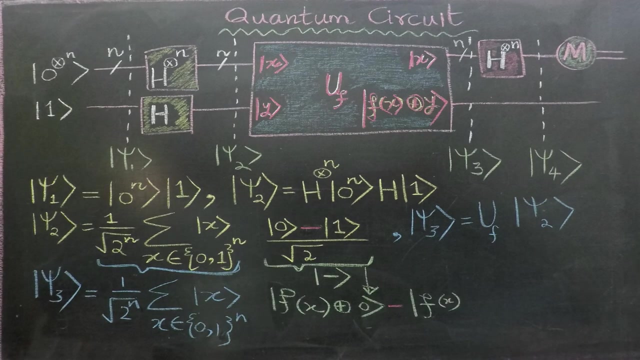 to the UF gate is ket x and ket y, The input will be ket x and ket f of x, solved with ket y. Thus, upon applying UF gate to ket psi 3, the first registers remain unchanged. where the second register is transformed to ket f of x- XORed, with ket 0 minus ket f of x XORed. 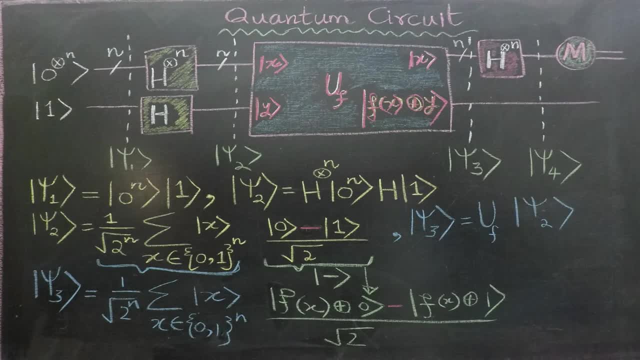 with ket 1.. F of x XORed with 0 is equals to f of x, whereas f of x XORed with 1 is the complement of f of x. We substitute these values into ket psi 4 to simplify it further. 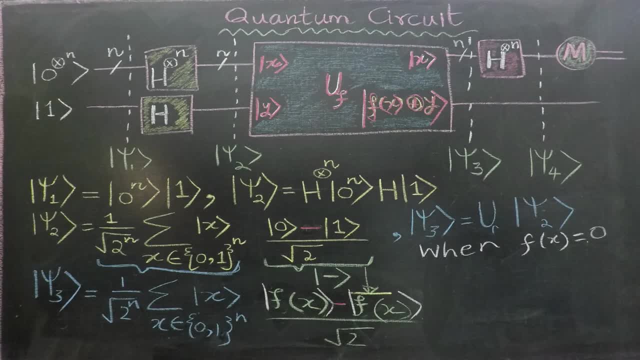 Note that when f of x is equals to 0, the second register will have ket 0 minus ket 1 divided by the square root of 2.. F of x XORed with 0 is equals to f of x, whereas f of x XORed with 1 is the complement of f. 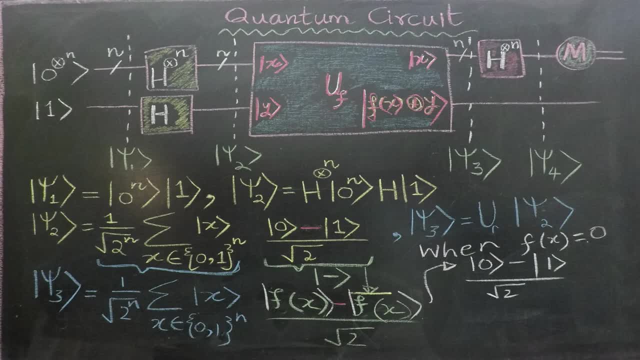 of x. This is what we mean by ket 1 minus the square root of 2.. In contrast, when f of x is equals to 1, the second register will have ket 1 minus ket 0 divided by the square root of 2, which is basically minus of ket minus. 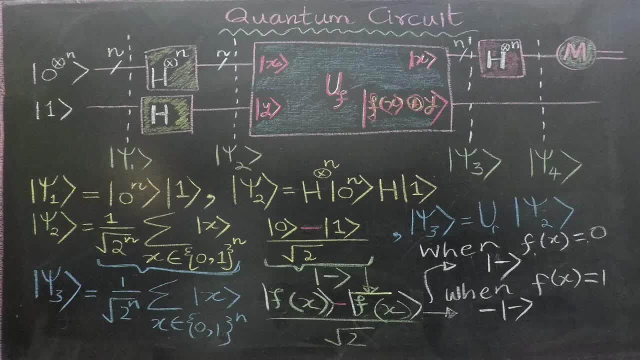 This shows that we will have a minus sign if, and only if, f of x XORed with 0. So if we do this, then the second register will have the same function as ket 0 minus ket 1.. only if f is 1.. Therefore, we can rewrite the second register as minus 1 raised to the. 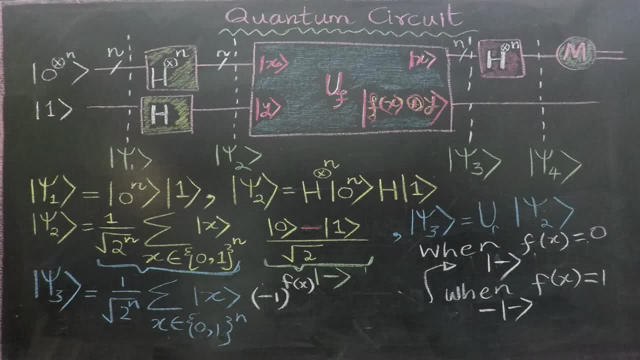 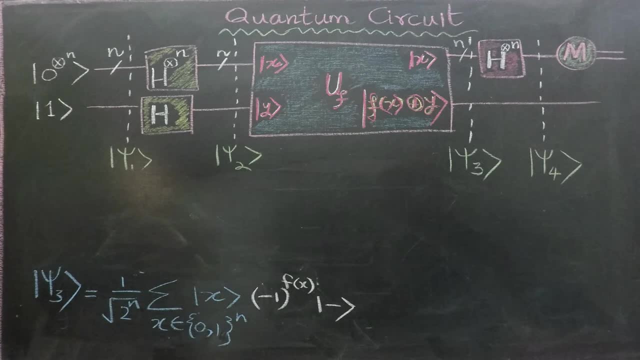 power f times ket minus. Let me clear the blackboard to make some space. ket psi 4 is calculated by applying the Hadamard gate on the first register only and keeping the second register as it is. In fact, we do not need the second register for our future. 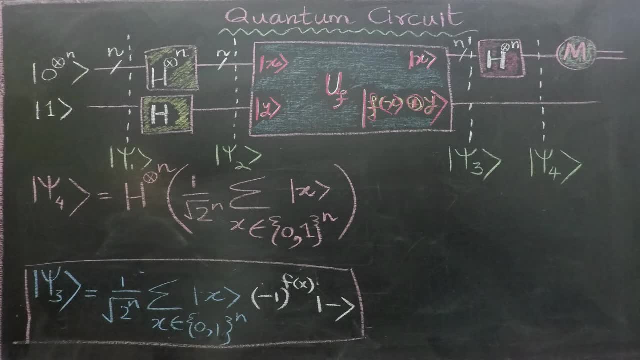 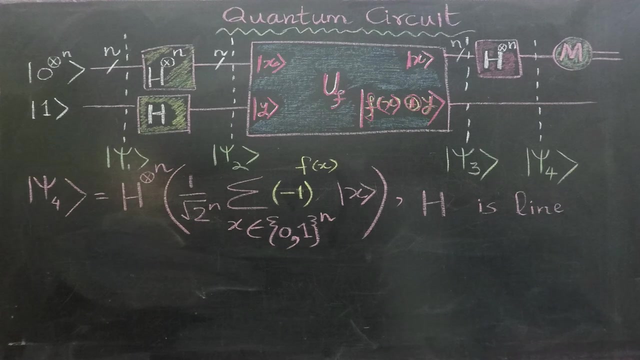 calculation, So I will not be writing it from here onwards. Oh, I forgot to include minus 1 raised to the power f in my ket psi 4.. Let me make this correction here. All quantum gates represent linear functions. Therefore I can take the Hadamard gate inside. 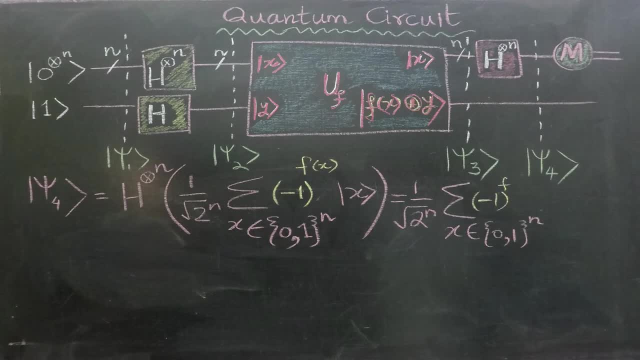 the summation and apply it on ket x, So I can take the Hadamard gate inside the summation and apply it on ket x. The application of Hadamard gate on ket x transforms it into an equal superposition of all n-qubit values of a variable y. The sign of these values depends on both x and. 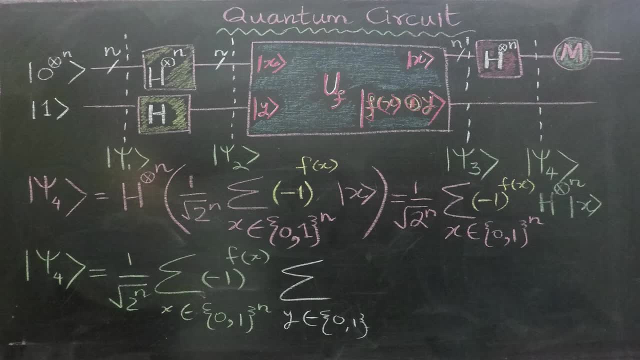 y. Therefore we can express it as minus 1 raised to the power x and y. If you still have any confusion in understanding the operation of the Hadamard gate, I suggest you watch my series of videos where I explain this gate clearly. 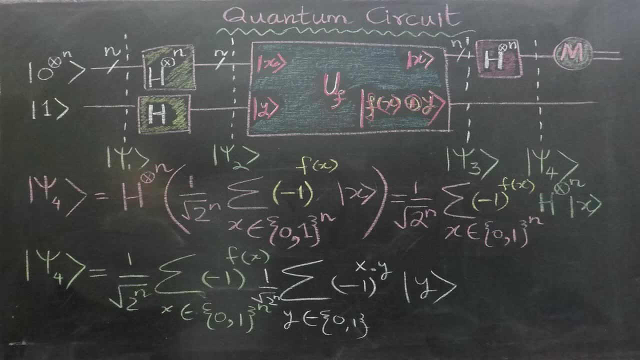 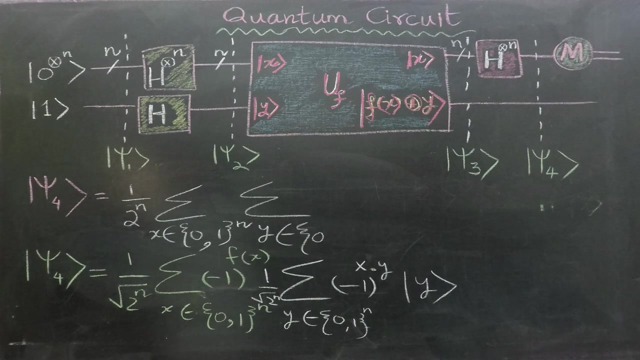 Anyway, to simplify ket psi 4, we rearrange the two summations. We take our both instances of 1 over square root of 2 and multiply them, resulting in 1 over 2.. Furthermore, we multiply minus 1 raised to the power f of x and minus 1 raised to the power x and y. This is the. 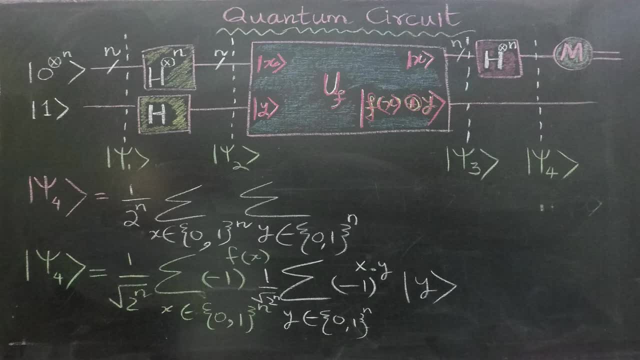 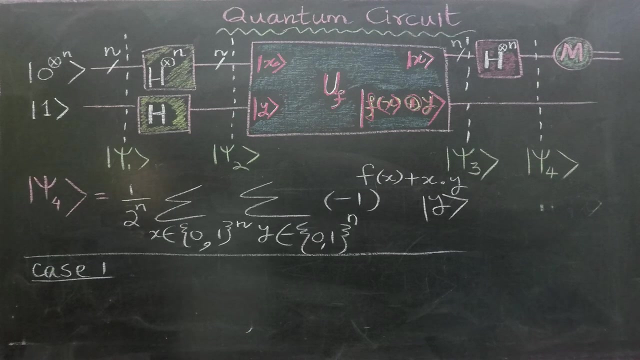 result of the addition of the two summations and we get minus 1 raised to the power f of x plus x and y. That's it, We are now ready to measure our first register. Consider a case where the function is constant. In this scenario, we claim that we can measure y as 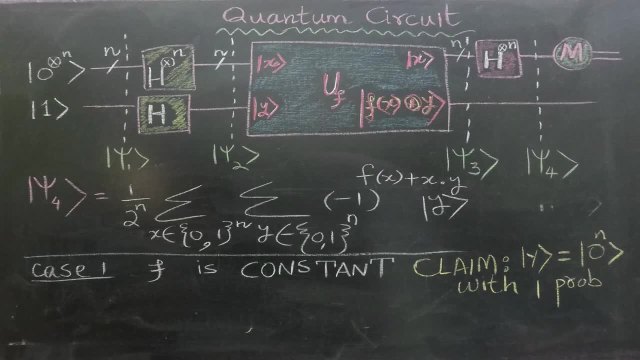 ket 0 with a probability of 1.. Let's verify this claim by calculating the probability of measuring ket 0.. Firstly, note that x and y will be 0, as y is ket 0.. With a constant function, we will either always get: f of x is equal to 0 or f of x is equal to 1.. If 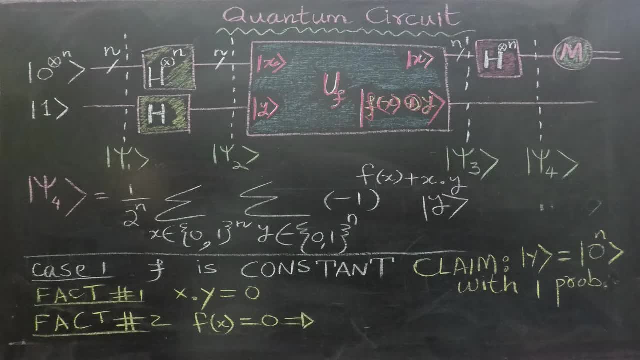 f of x is equal to 0, then minus 1 raised to the power f of x will always return 1.. Thus in the numerator we have the summation of all 1s raised to the power x and y We. 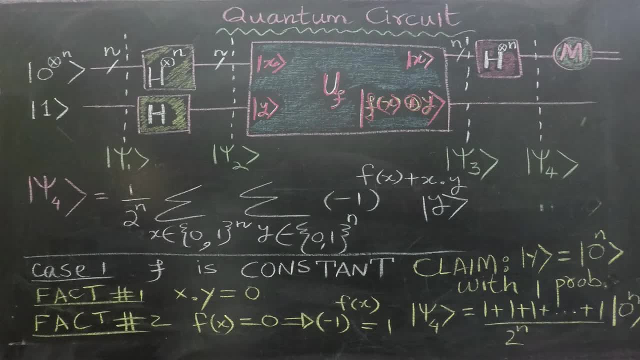 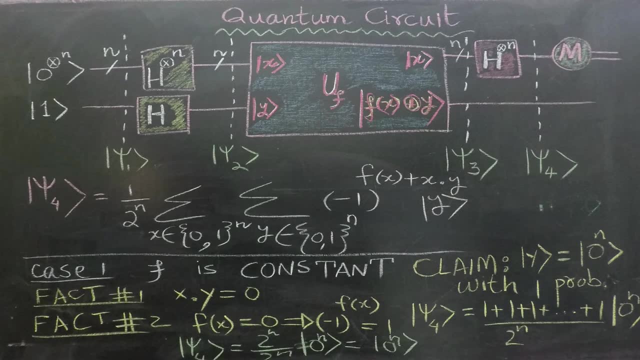 write it as: f of x is 1.. Therefore we have: f of x is equal to 0, and f of x is equal to 1.. By CAD 0, we get f of x is equal to omega square times the number of functions. 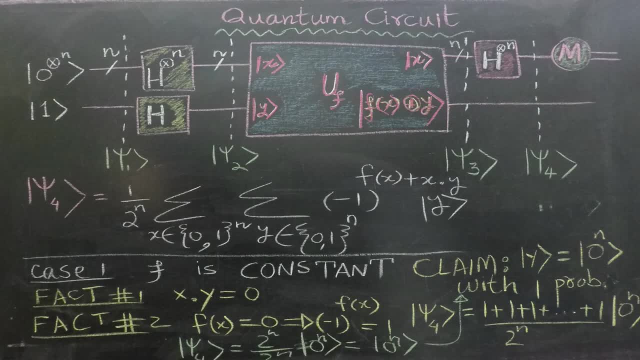 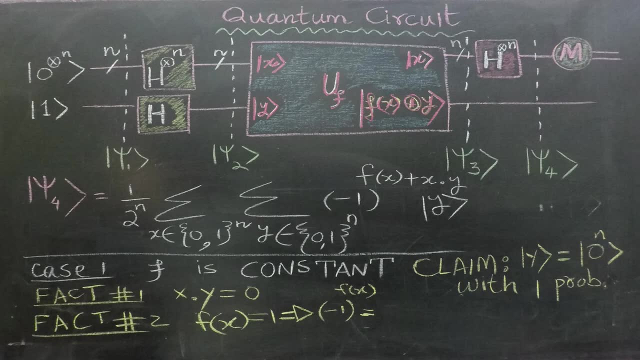 that are present in the two substitutes of f of x and x. In contrast, when f of x is equal to 1, then minus 1 raised to the power of f of x will always return minus 1.. Thus in the numerator we have the summation. 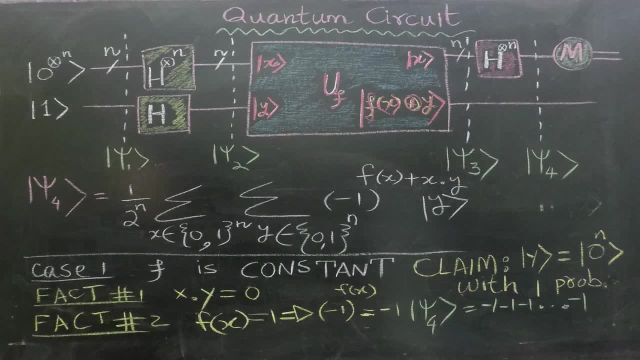 all minus 1s, resulting in minus 2. raised to the power n, The numerator and denominator cancel each other, making the amplitude of measuring cat 0 equals to minus 1.. Scaling this amplitude of minus 1 will once again gives us 100% probability of measuring y is. 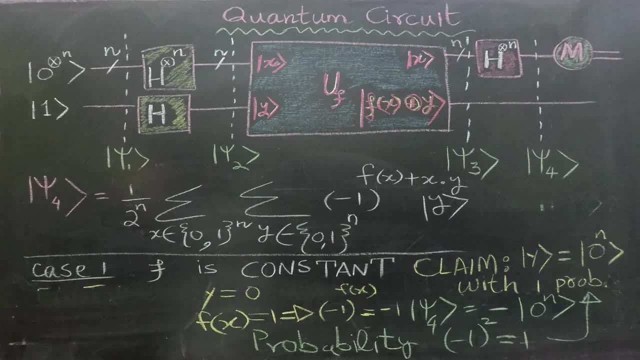 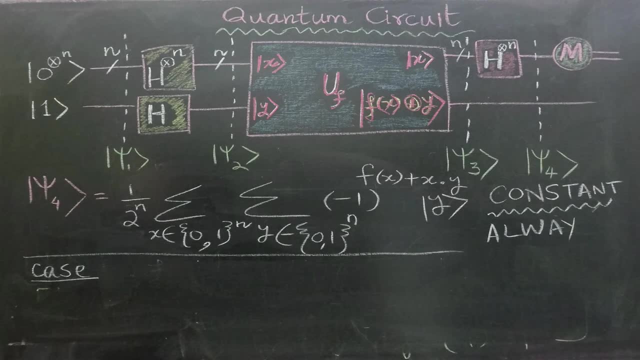 equals to cat 0.. In conclusion, when the function is constant, for both f of x is equals to 0 and f of x is equals to 1, we will measure: y is equals to cat 0 with 100% probability. So we have verified our claim. Now consider the case when the function f is balanced. 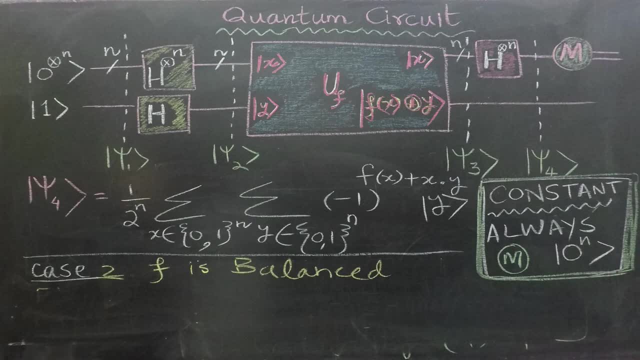 The claim is that in this scenario we will never measure y is equals to cat 0.. Let's verify this claim by computing cat 0. Let's see if the probability of measuring cat 0 is 0 or not. Once again, x and y will be 0, as y is cat 0.. When f is a balanced function, then half. 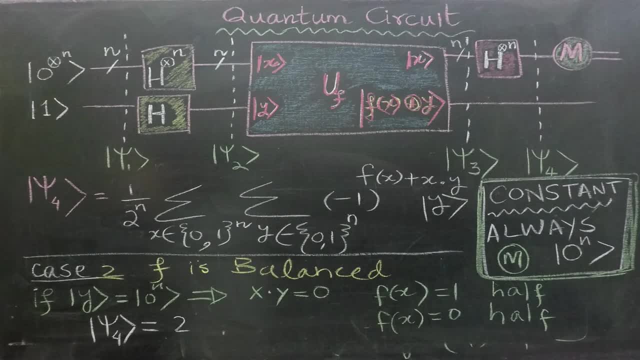 that is, 2 raised to the power n minus 1 of its input will return minus 1, and the remaining half, 2 raised to the power n minus 1, will give an output of plus 1.. This means the summation will return minus 1.. 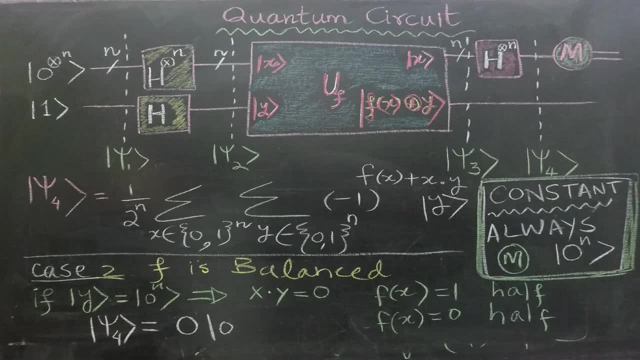 We can see that f is equal to 0. when f is a balanced function, The zero amplitude when scaled gives us a zero probability of measuring. y is equal to cat 0.. In conclusion, when the function is balanced, we will never be able to measure. 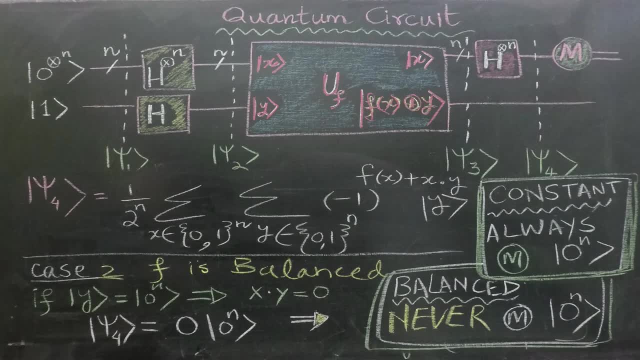 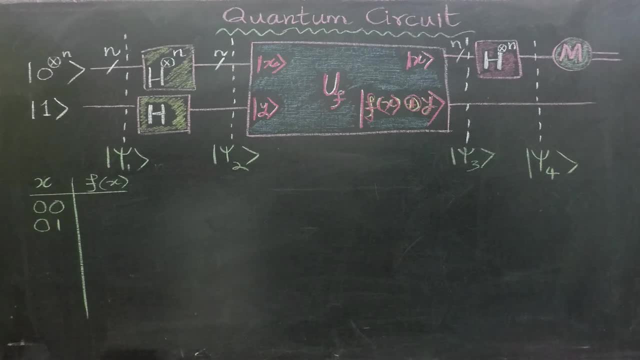 cat 0. Hence we have verified our claim once again. Let's consider an example in which n is equal to 2.. The function f is balanced in this example. The function f is balanced. in this example, The function returns 1 on input 2.. So this: 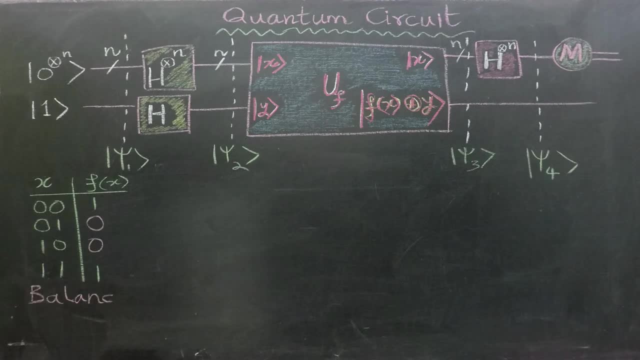 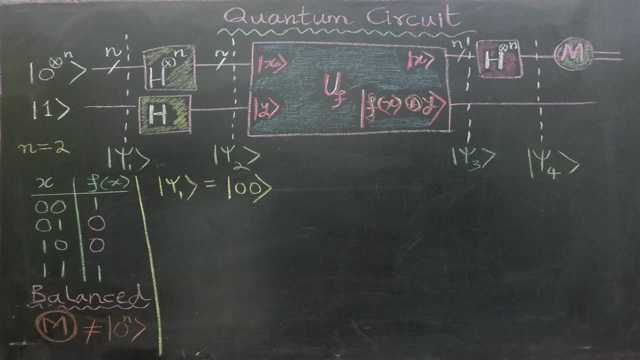 is the function. f is balanced. Now let's think about the fully balanced function. If we compute this function, perhaps zero, zero and one, one, otherwise it returns zero. cat psi one will be equals to tensor product of cat zero, zero and cat one. 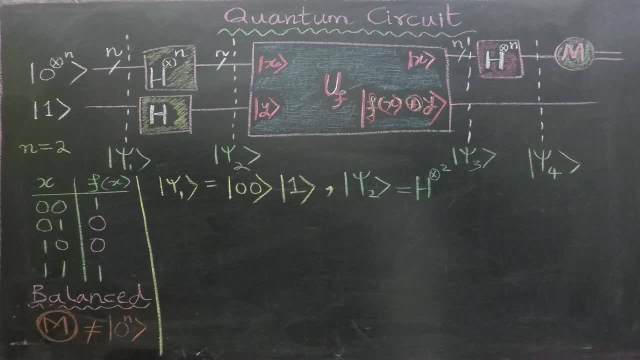 In cat psi two. we apply Hadamard gate to the both registers. The first register transformed into one over two times cat zero zero plus cat zero, one plus cat one, zero plus cat one one. The second register will have cat minus. In cat psi three. we apply Uf gate two the registers sense. the second register has